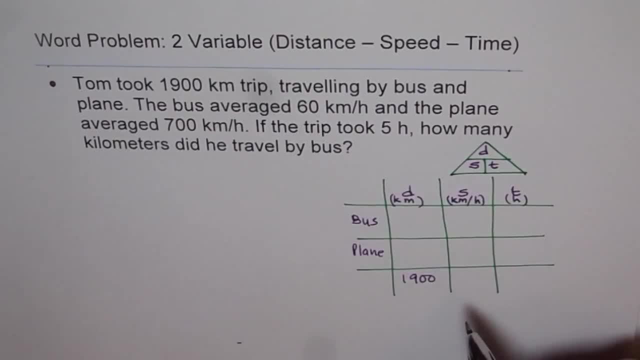 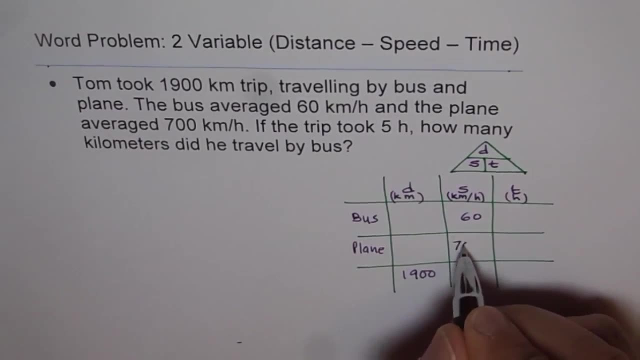 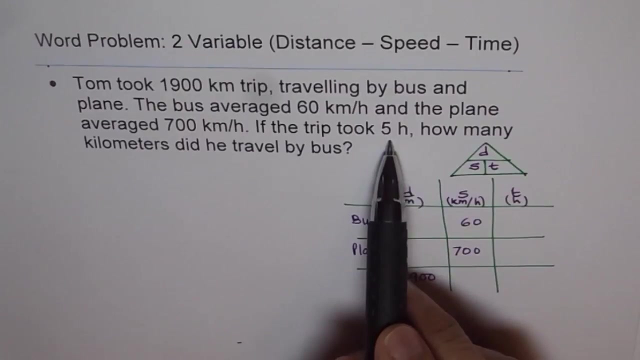 So that is our table. So then let us take the total distance covered by bus and plane, So we will put kilometers. the bus averaged 60 km per hour and the plane averaged 700 km per hour. So that is the speed: Sixty kilometers per hour for bus and 700 kilometers per hour for the plane. If the trip took 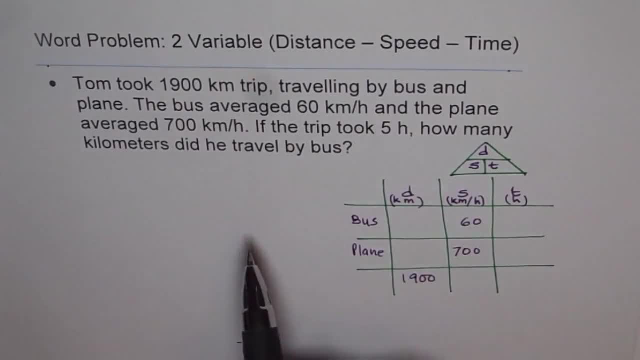 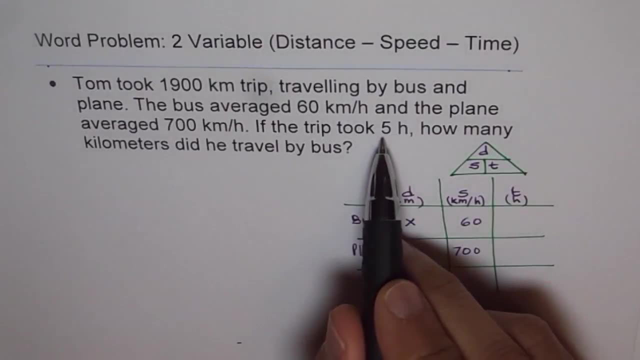 5 hours. how many kilometers did he travel by bus? So how many by bus? That means variables. So we will put x kilometers by bus And total trip time is 5 hours. So we are going to put the total distance and that is our table. So let us keep the table and then we will look at the table one by one. So we 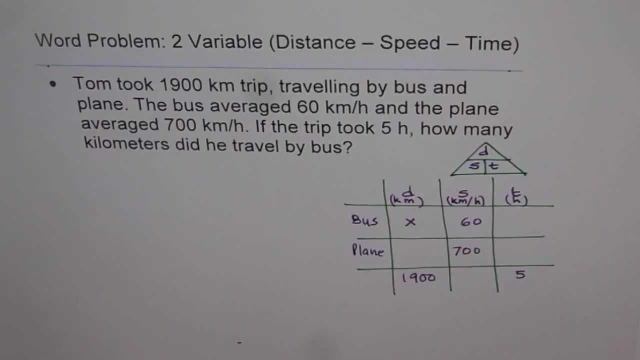 So we'll write total time here. so that is our total right. So whatever we'll do, we'll write sum or total here at the end. So total time is 5 kilometers for us. Now let's get back to the question and define our variables. 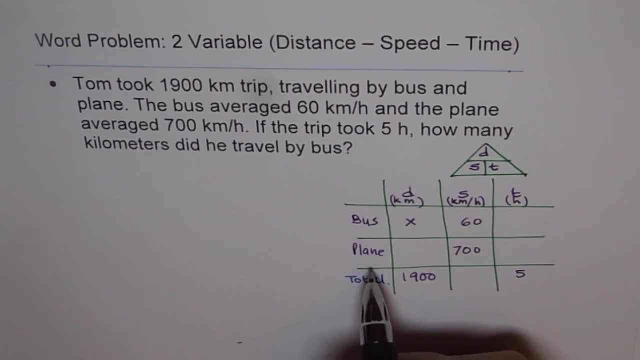 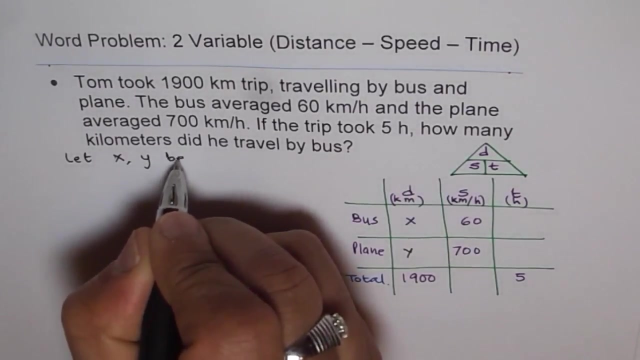 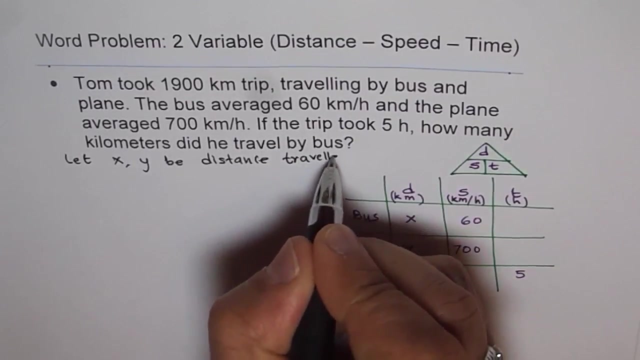 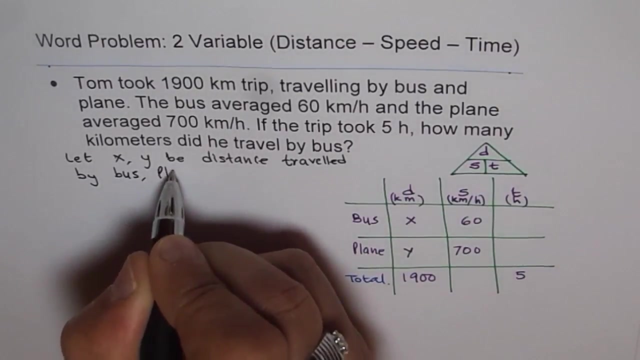 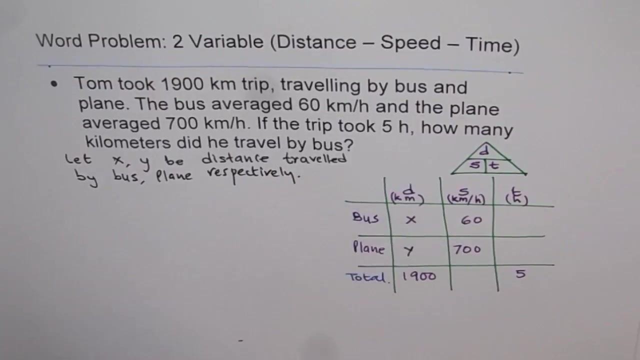 Now the variable here is: let X be the distance traveled by bus and let Y be the distance traveled by plane. So that is our variable. So let's statement is: let X and Y be distance traveled by bus and plane respectively. So we have defined our variables. 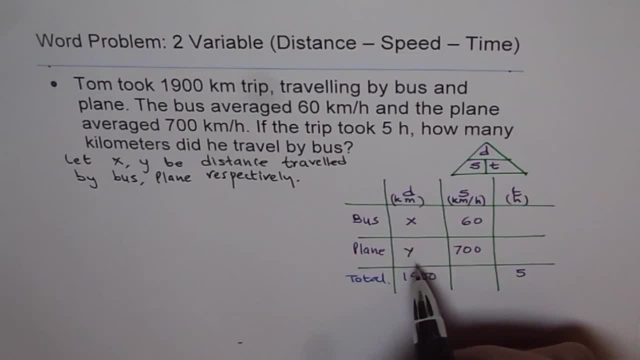 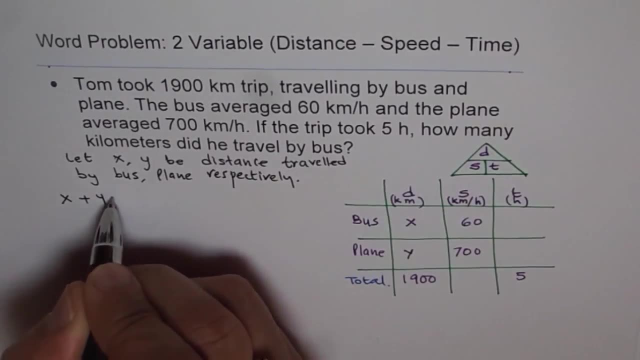 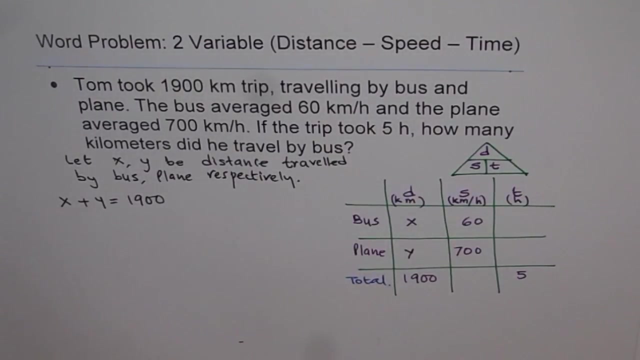 Okay, Now we can figure out the relation between them. Relation is: X plus Y is 1900, since that is the total distance, right? So X plus Y equals to 1900.. So when we have two variables, it's a good idea to write one in terms of another. 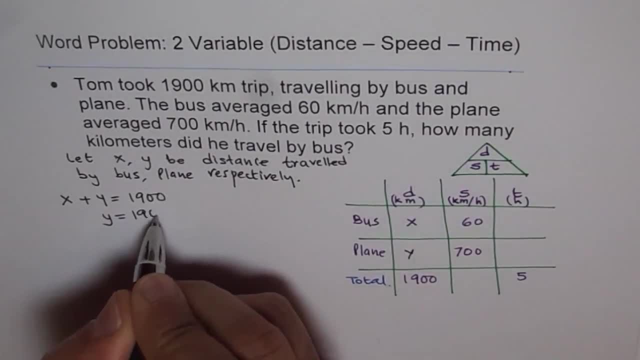 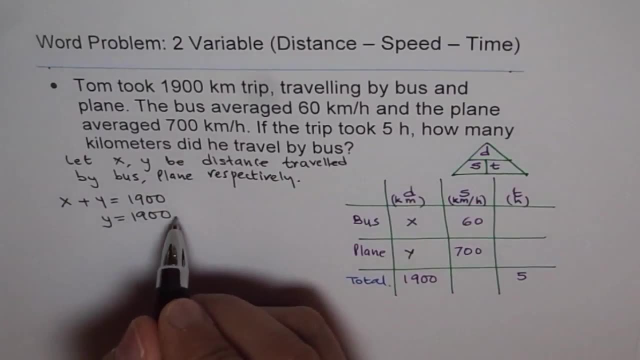 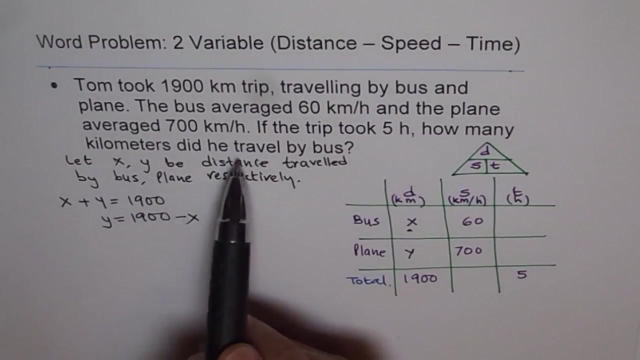 So we can write from here: Y equals to 1900.. We are writing in terms of Y: Y equals to 1900 minus X, Since we want X to be there, right? This is what we want to know: How many kilometers did he travel by bus? 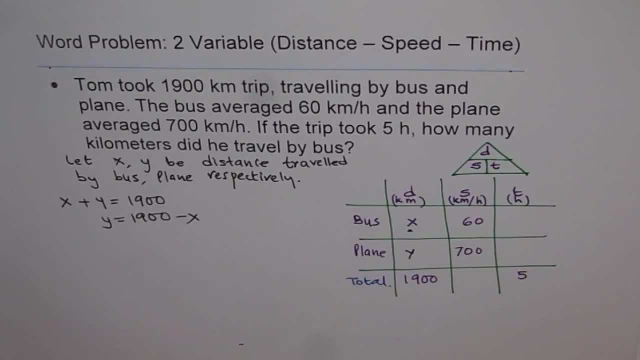 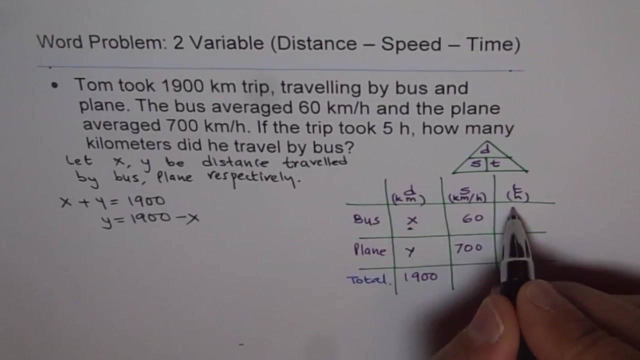 So we'll get equation in X, We'll solve for it and get our answer. Now time From this relation we know time is distance divided by speed. So time taken during this trip by bus will be how much Distance of X divided by speed, which is 60.. 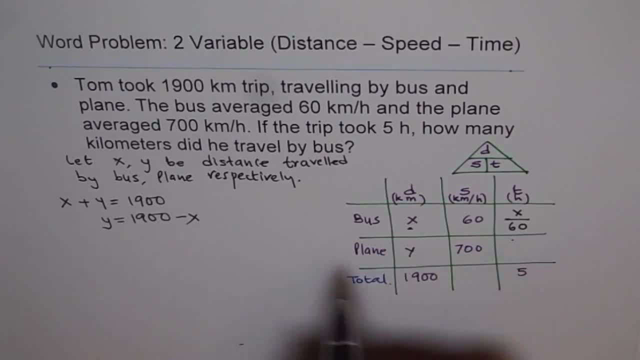 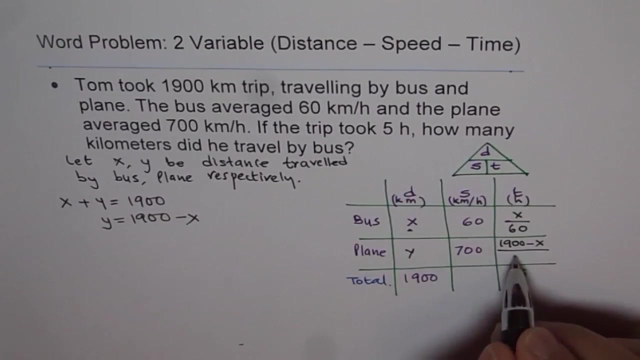 How about? plane Distance of Y and Y? for us is 1900 minus X, So instead of Y I'll write 1900 minus X. So we have 1900 minus X. Total was 1900.. So Y is 1900 minus X divided by the speed of 700, right? 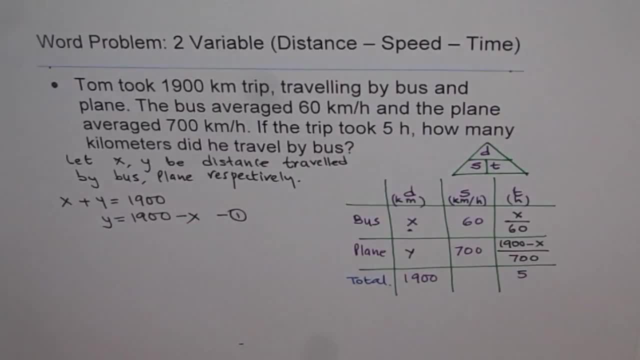 So we have used equation 1 here to relate distance traveled by plane with distance traveled by bus. Now you notice, if you add these two times you should get 5 hours, since the total time taken is 5 hours for the trip of 1900 kilometers. 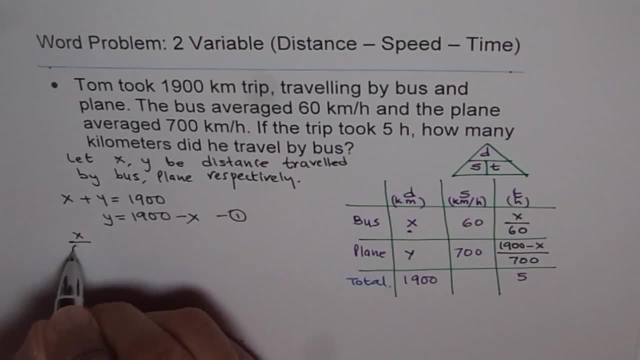 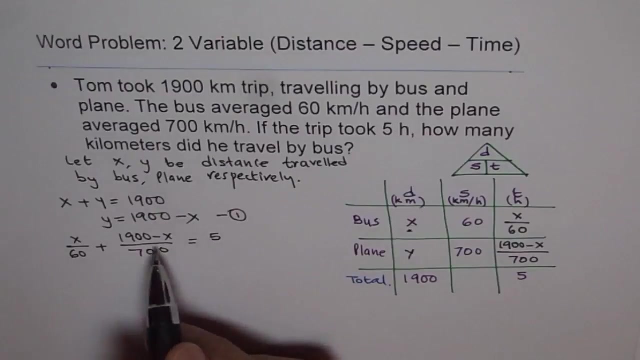 So we get our equation, which is X over 60 plus 1900, minus X over 700, and that should be equals to 5,. okay, Now we can take common denominator. We can take common denominator and solve for X. So the common denominator here is 4200, 7 times 6 and then 4200. 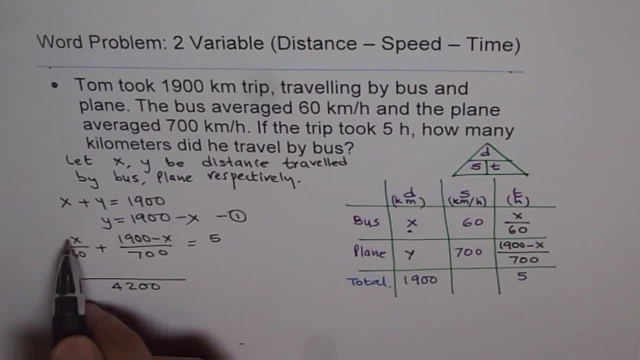 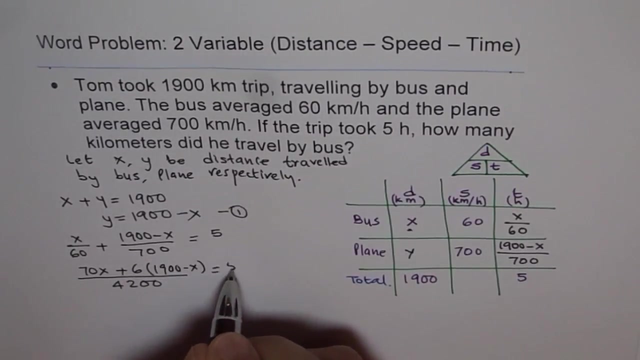 So to get 4200, we need to multiply this by 70, right? So we get 70 times X plus, and this should be multiplied by 6,. 6 times 7 is 42, 4200.. So 6 times 1900 minus X equals to 5, correct. 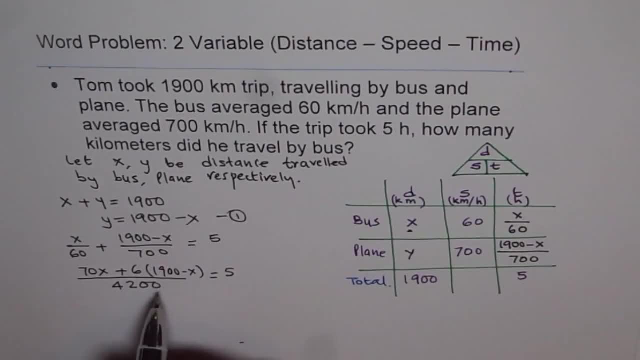 So we can use this, So we can use calculator. multiply all this and then we'll multiply both sides by 4200 to get rid of fractions. So let's do that, So we get 70X plus 6 times 1900.. 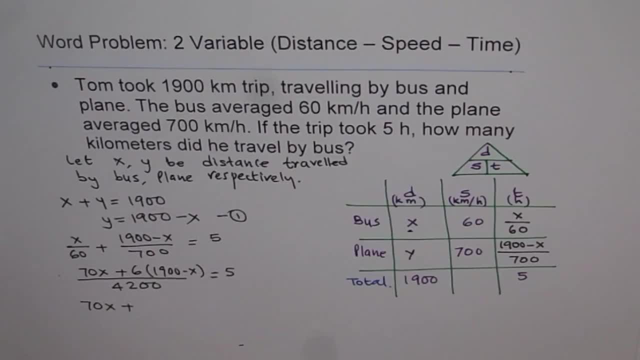 Let me use the calculator now: 6 times 1900 is equal to 11400.. So we get 11400 minus 6X equals to 5 times 4200. Okay, Okay. Now this 70X minus 6X will give us 64X equals to. we'll have here 4200 times 5, which is: